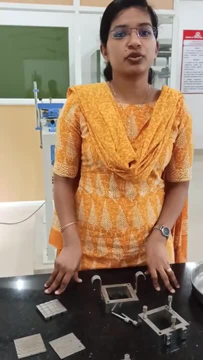 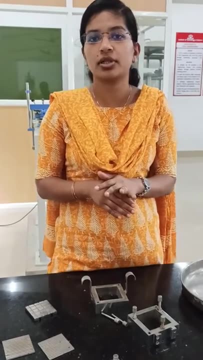 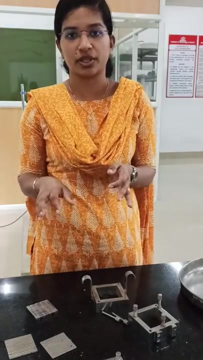 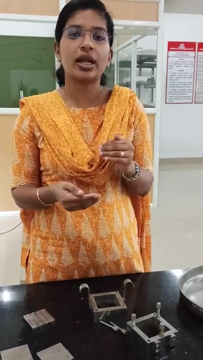 Good morning students. So today we are going to see a test for determining the shear strength of the soil. So we have learnt in our theory course that shear strength is an important parameter of soil. So the shear strength of soil is its capacity to carry the shear loads coming over it. So in order to test the shear strength of the soil, we have four different tests and this test will help us to determine the shear parameters of the soil. So shear parameters means it is 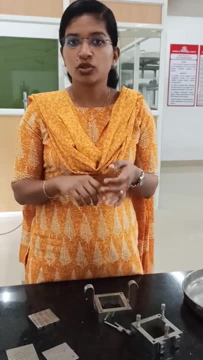 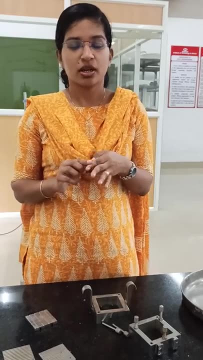 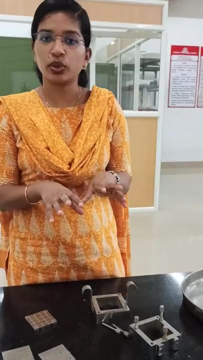 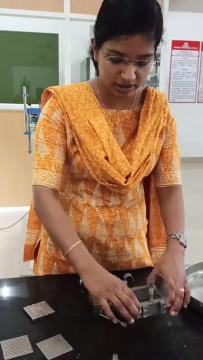 cohesion C and angle of internal friction, phi. So from these four set of tests- that is, we have triaxial test, we have UCC test, direct shear test and wane shear test- From among these tests we will get the shear parameters of the soil. and among these four tests we are doing the first test, that is, direct shear test now. So for that we have a shear box. This is a shear box. This shear box is having two halves. Okay, this is a low. 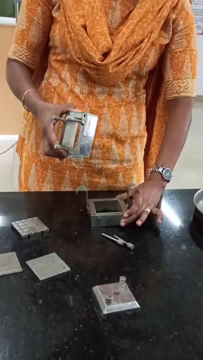 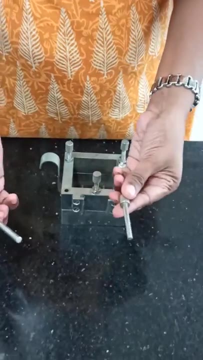 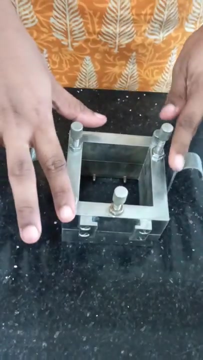 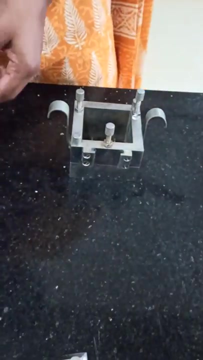 half, and this is the upper half. So the upper half is placed over the lower half, and these two are the locking screws, and here we have the hole for locking screw, and when we tight this locking screw, then this act as just one single box. Okay, So along with that we have a grid plate or a base plate here. This we should keep at the bottom most. 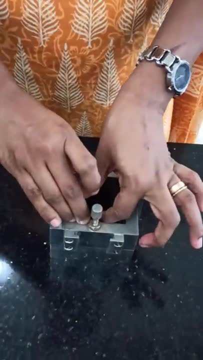 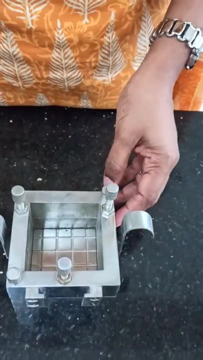 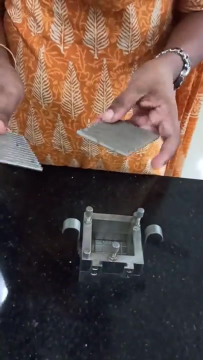 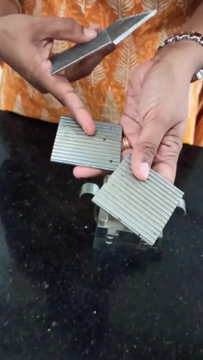 portion. Okay, So I have placed the base plate. Now another thing. I will say friction plate or grid plates. we say So this. grid plates are of two types. They may be porous grid plates or non-porous grid plates. Okay, So this porous grid plates we use, or this porous friction plate. 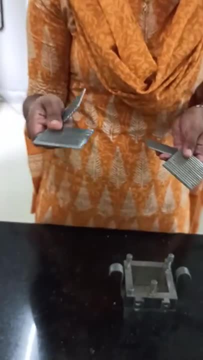 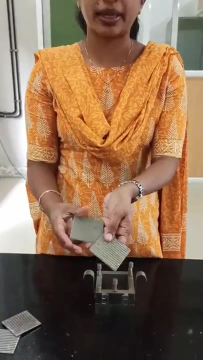 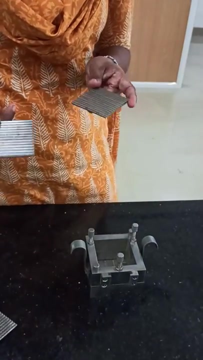 plates we use when we have to do a drained test, wherein we allow the drainage of water, we permit the drainage of water and this non-forest one or the plain plates we use for undrained test, okay. when we do not allow the drainage of water, we use a plain plates, okay. so 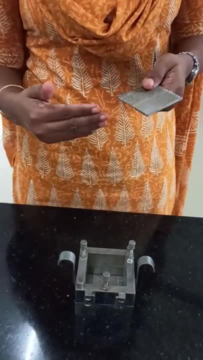 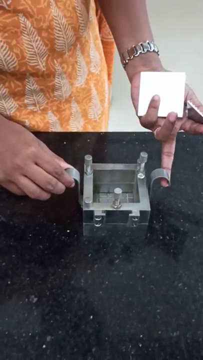 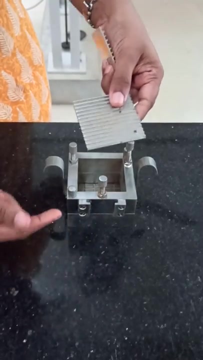 this plate. we have to keep in a direction perpendicular to the direction of action of shear force. okay, so, here you see, in this shear box, we are applying the load from this direction. horizontal load is applied from this direction, so we should keep the grid. 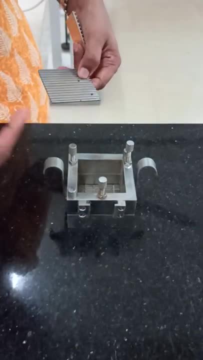 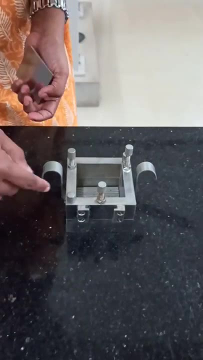 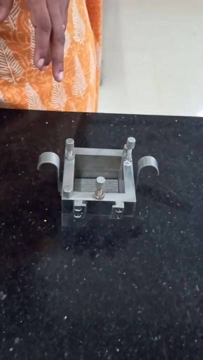 plate, such that these lines of the grid plate should be perpendicular to the direction of application of shear load. okay, so one plate should be placed at the bottom. now, after this, we have to fill soil into this shear box. okay, Whichever soil we require for the test, or whichever soil we have collected for the test. 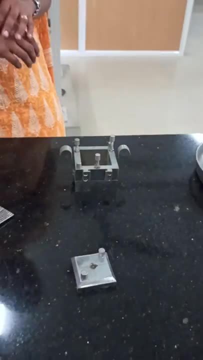 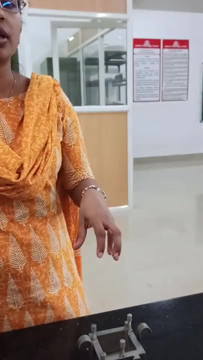 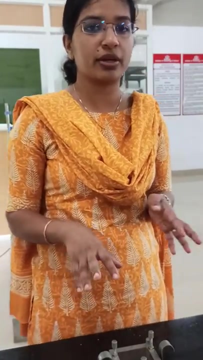 we should fill in this shear box, so for that we may be given a specified density with which we have to fill the soil into this and suppose, if that density- I am taking here that density- as to 0.5 kilogram per meter cube, so with that density I have to fill the soil in this. 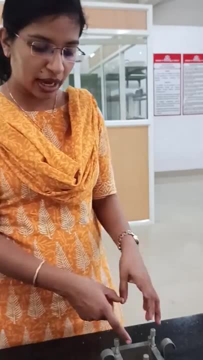 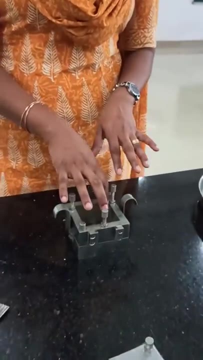 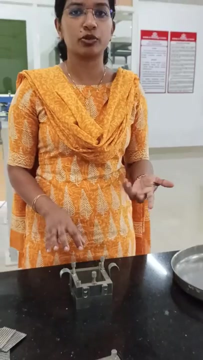 apparatus or the shear box. So I have to know the volume of this shear box. from this, just measuring the dimensions of this shear box, I will get the volume of this shear box and the density of filling required is given to me. with that volume and density of filling I will calculate the amount. 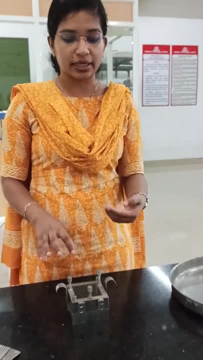 of soil or the mass or weight of soil which is to be collected for filling into this. okay, So I should fill the required density of the shear box, okay. Okay, So I should fill the required density of the shear box, okay. 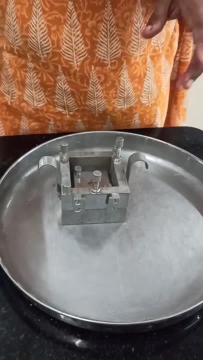 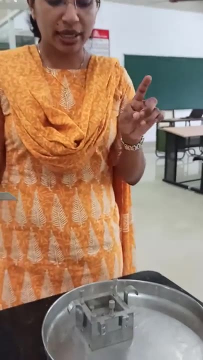 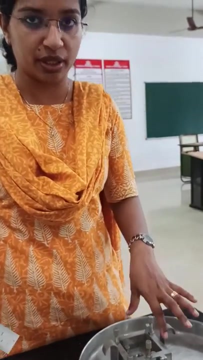 Okay, Required soil into this shear box into this specified density. We have to fill this into the specified density So that specified density into the volume of the shear box to be filled. That gives the mass of the soil which I should take for this. 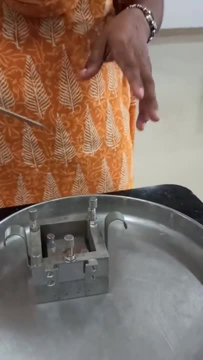 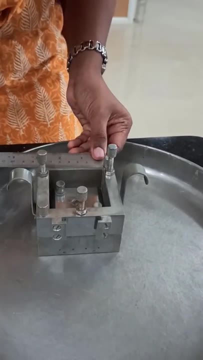 So now I am going to measure the dimension, or measure the dimensions through which the soil is to be filled. So for that you measure the sides of this shear box. From that you will get. the one side of this shear box is 6 cm. 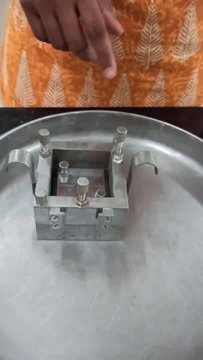 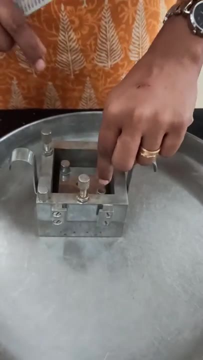 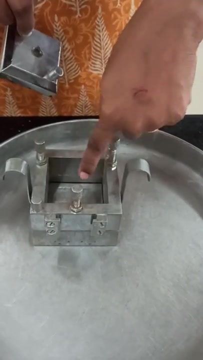 And this is a square shear box, and so that dimension is 6 cm. Now the height of filling: The height of filling should be obtained after placing this loading pad as well as the second plate grid plate. I have placed the second grid plate here. 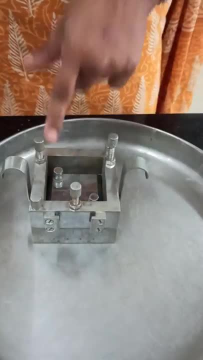 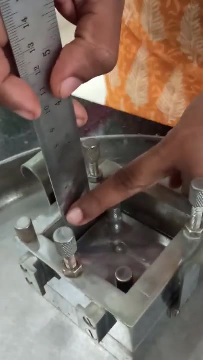 And the loading pad inside And the space remaining will be the space of filling of soil. So what is the height of that filling? So that height of filling is 3 cm. So 3 by 6 by 6 is the volume of filling of soil. 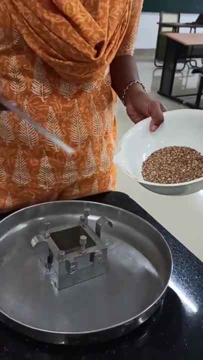 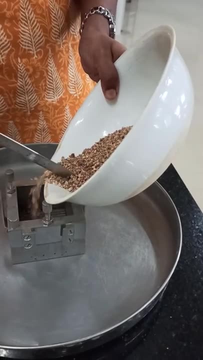 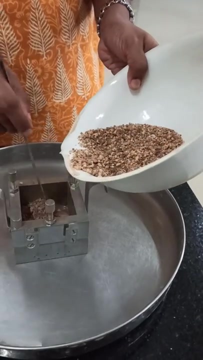 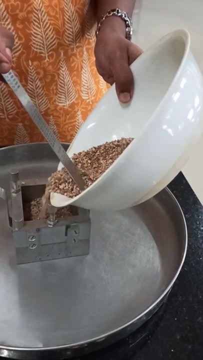 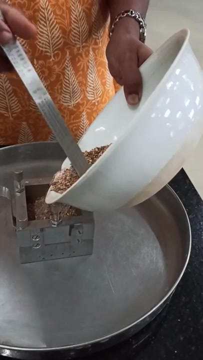 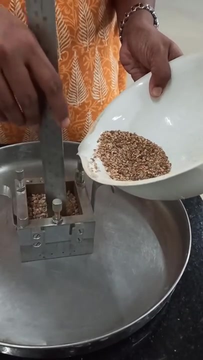 Now I have measured the required quantity of soil which is required for filling. So carefully, fill that soil into this apparatus. So here, this is the matrix. So here, this is the matrix of soil, And this is the pipe, And this is the pipe. 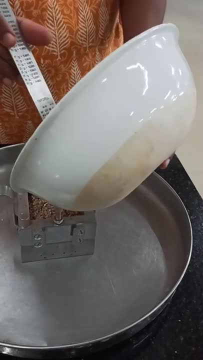 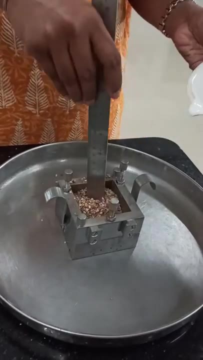 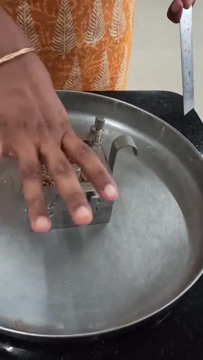 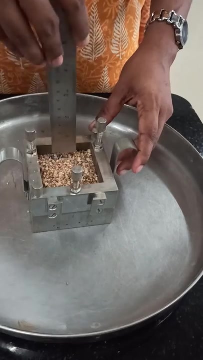 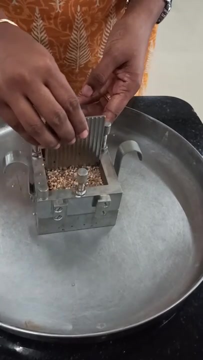 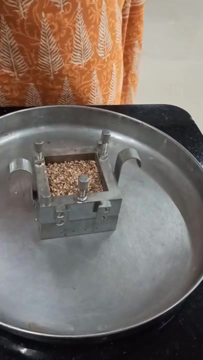 And this is the pipe. So let's start. So let's start with the surface and place the second grid plate or friction plate. Okay, So again, when you place the friction plate, you should see that the lines of the friction 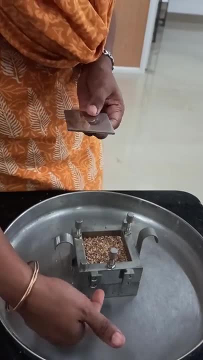 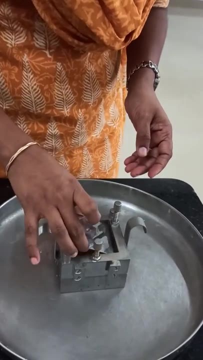 plate should be perpendicular to the direction of action of shear force. So this is the direction of action of shear force. So the lines should be like this, such that it is perpendicular. So place it, And over this we are placing a load. 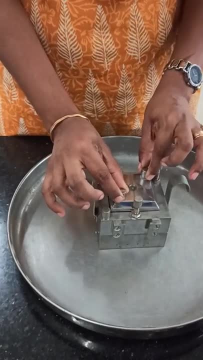 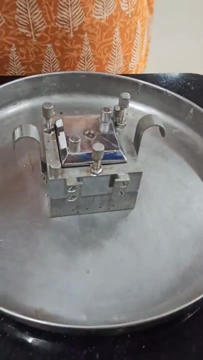 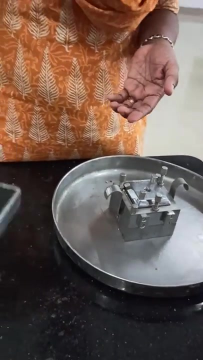 Loading pad. This is the loading pad of the apparatus and that should be placed here. Okay, So this is how we fill the soil into the shear box. Now we have a extruder here In case, if we are taking the soil directly from the field, you can insert it into the. 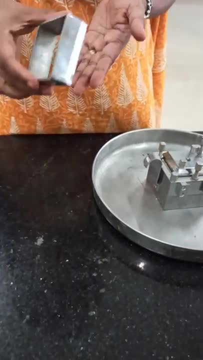 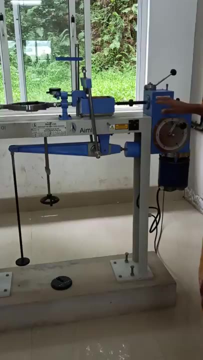 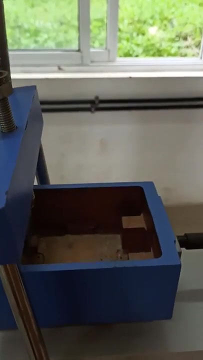 field soil and the soil will be filled into this And that soil you can directly transfer to the shear box. So this is the shear apparatus. So for this we have a container here. So this is the container where we keep the shear box, which is filled with soil. 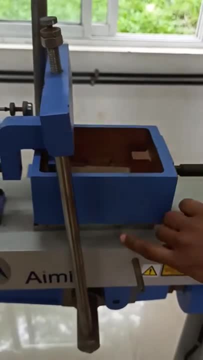 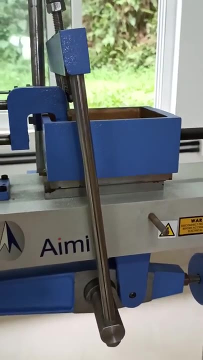 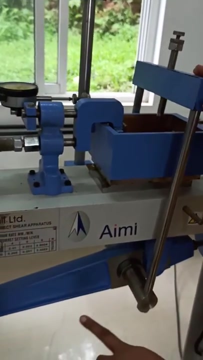 We keep in this container, So this is a movable container. On basilar, there are balls over which this entire container will move. Okay, Now, after that, this is the loading frame. This is a loading frame, So we keep the load here. 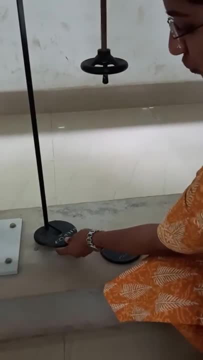 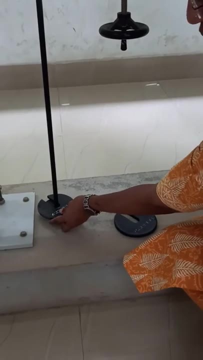 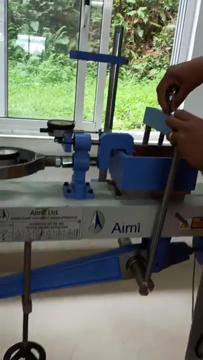 So this is the load we have. This is a load which is of 0.1 kilogram per centimeter square. Okay, So when we place this load here, this will be transferred through this lever onto this loading frame and that load will act on this soil which is placed here. 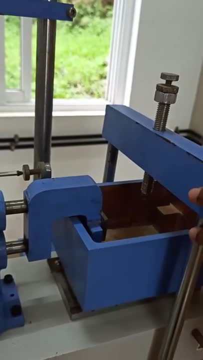 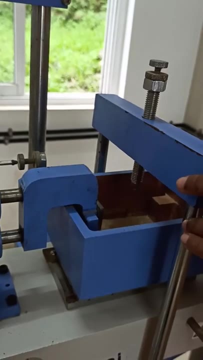 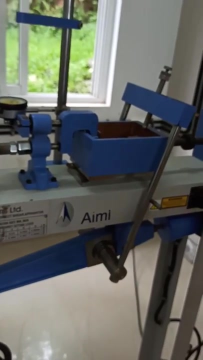 Okay, So that load will be transferred such that it gives a stress of 0.1 kilogram per centimeter square normal load over this. So that load will be transferred to this particular soil sample. Now we may give a stress of 0.1 and then we may vary the stress as 0.2, 0.3 and so on. 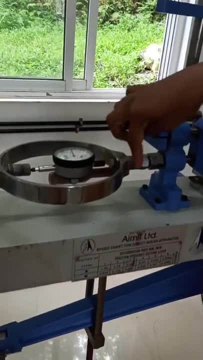 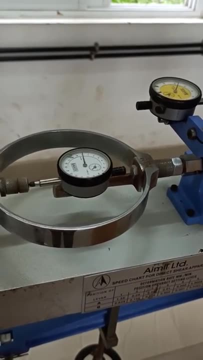 Okay, So then we have a proving ring here. This is a proving ring for measuring the load which is coming, horizontal load which is coming on this soil sample placed in the container. Okay, So the movement of this ring, needle of the proving ring, indicate that the load is coming. 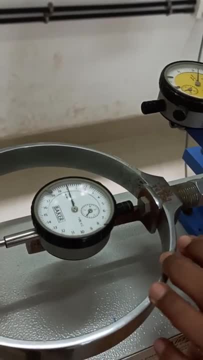 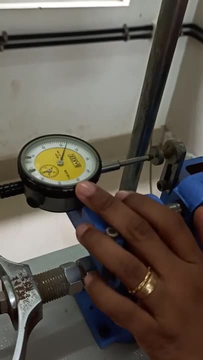 Okay, So this is the loading frame. So this is the loading frame. Okay, So this is the loading frame. So this is the amount of shear load. And again here there is a dial gauge which measures the amount of displacement horizontal. 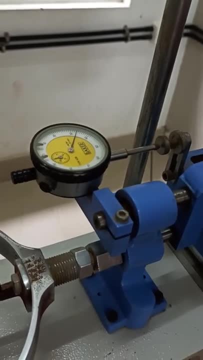 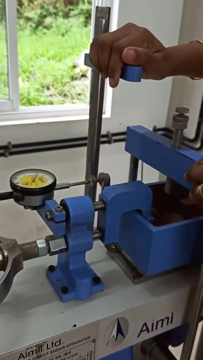 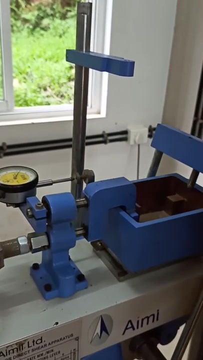 displacement which is happening here on this box. Now, if we have to measure the vertical displacement, we can attach a dial gauge on this and we can connect it to the shear- I mean load frame- so that we can measure the vertical displacement also. 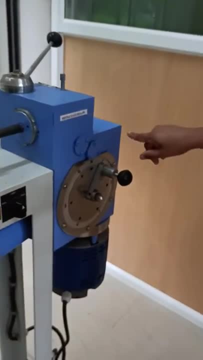 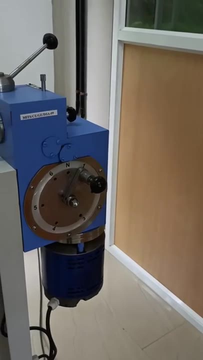 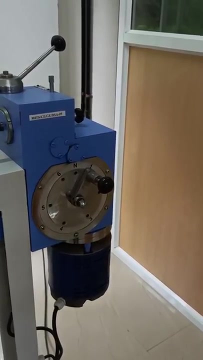 Now here There is a level here. So this shear test is done generally as a constant strain test. So the strain which we apply is usually we apply or for this test we apply it as 1.25 mm per minute. 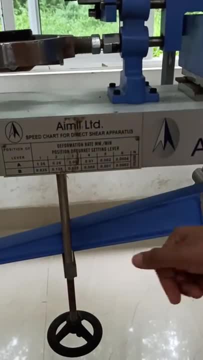 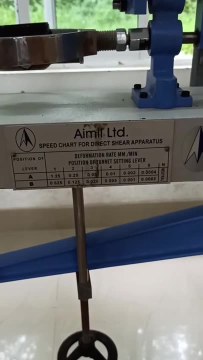 So you can see the table chart here. So when we place the lever at position A and 1, it corresponds to 1.25 mm per minute. So you see, here there is 1.25 mm per minute. 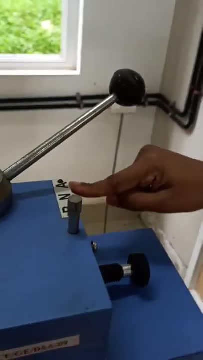 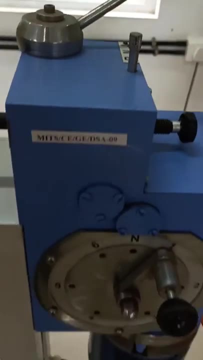 Okay, So now we can see the strain. here There is a position A and B for this liver and a neutral position. So when I place this liver to A and adjust this liver to 1, I get a strain of 1.25.. 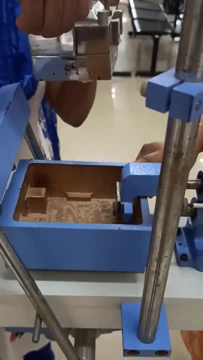 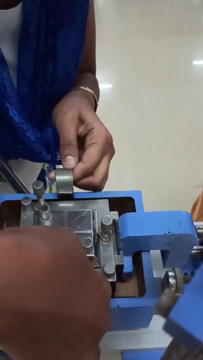 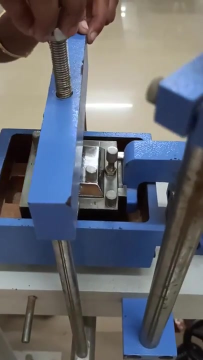 Okay, now we are placing the shear box into the container on the shear testing apparatus. This is how we place: carefully place such that no much displacement is given to the box. Now we have placed the shear box into the container. Now adjust the loading frame such that the screw touches the loading pad. 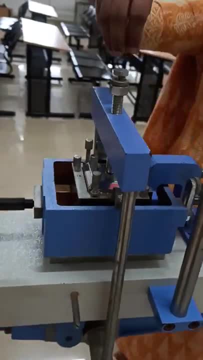 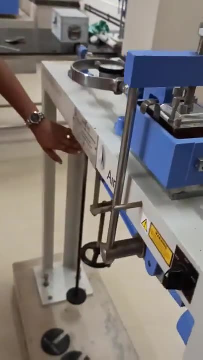 Okay, ensure that it just touches the loading pad. Do not give more stress on this. Okay. So next we have to see there is a liver arm here. Okay, we have a liver arm which transfers the load which we apply here to the box there. 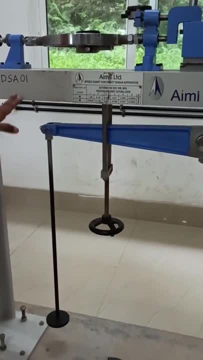 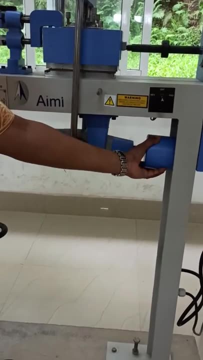 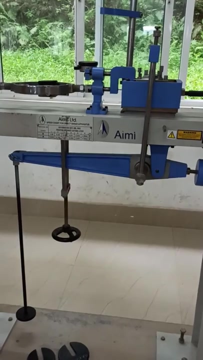 So this liver arm should be perfectly horizontal once we apply the load. So if in case it is not horizontal means we can adjust it to here. By turning this you can adjust the horizontality of the liver arm. So once it is perfectly horizontal, you apply the load. 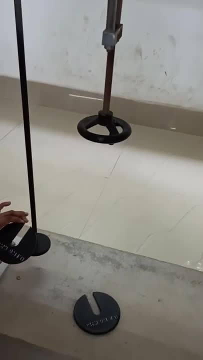 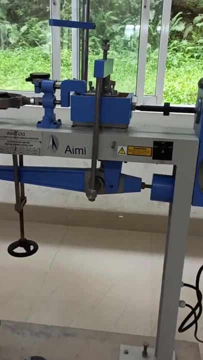 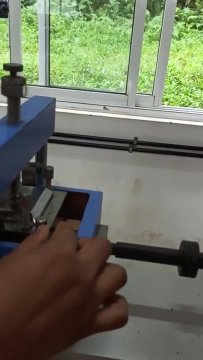 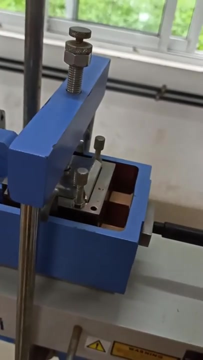 So initially I am applying a bar such that it applies a load of 0.1 kilogram per centimeter square over this shear box, Okay, and then you can remove the locking screws here. We have two locking screws here, So remove this locking screws such that the upper and lower plate of the shear box is free to move. 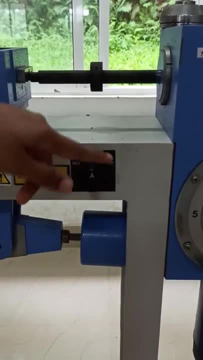 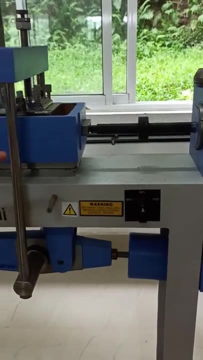 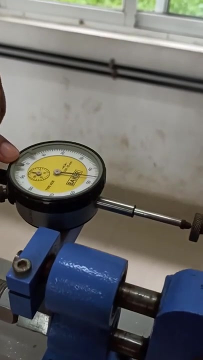 We can start the apparatus. For starting the apparatus, turn this, This knob to forward. You see, this is reverse and this is forward. So then, when we place it forward, the apparatus is started. So when the apparatus is starting this, you see this, there is a horizontal dial gauge which we have placed here, which measures the horizontal displacement. 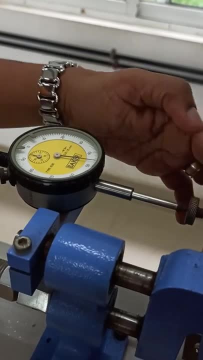 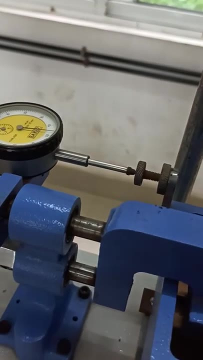 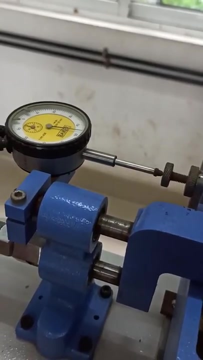 Now this dial gauge. at present it is not touching this shear box here, or the container is exactly not touching this shear box here. So initially there will not be any displacement. So the testing or the reading should be taken only after that initial touch is established. 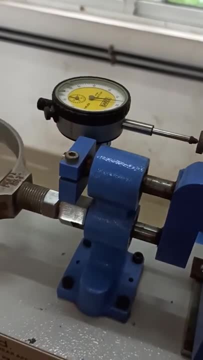 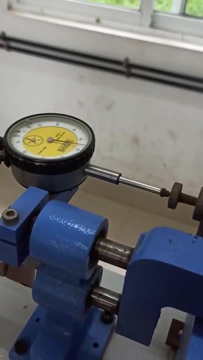 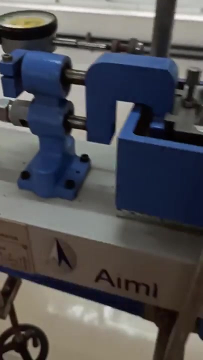 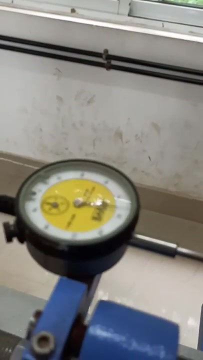 Okay, so for that, once you rotate the knob to forward, you should wait for the dial gauge to just start moving. So once it just starts moving, you should switch off the apparatus and set both these dials to 0.. Wait for the dial gauge to move. 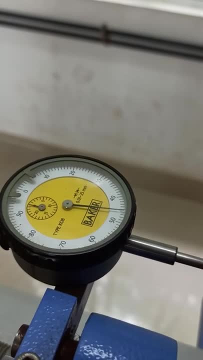 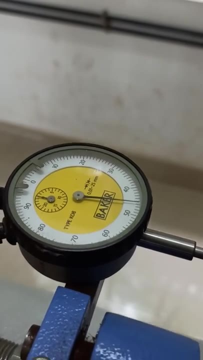 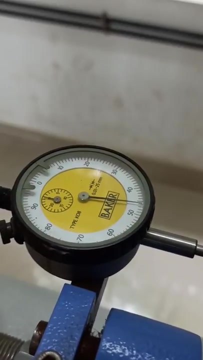 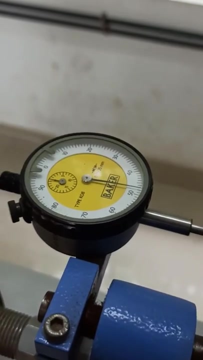 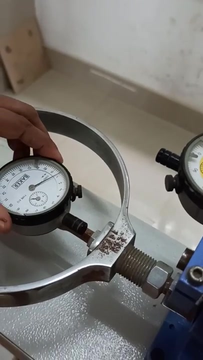 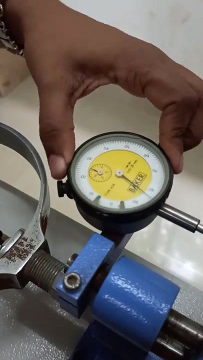 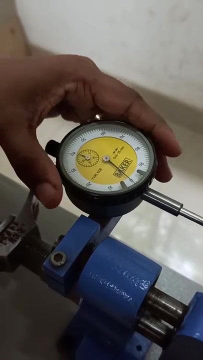 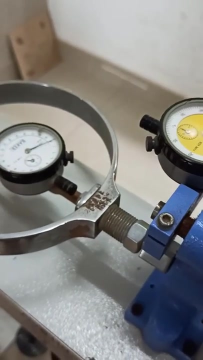 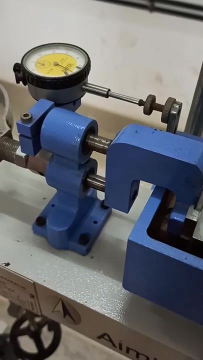 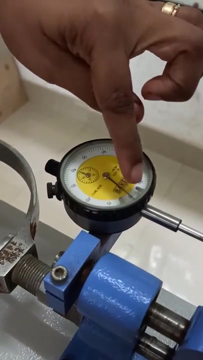 Wait for the dial gauge to move. Okay, now it started moving. Switch off the apparatus. Set both these dial gauges to zero. Now, both these are set to zero. Now you can start the apparatus to measure the load and displacement. So for every 20,- you can see here when the needle reaches 20, then 40,, 60,, 80 and so. 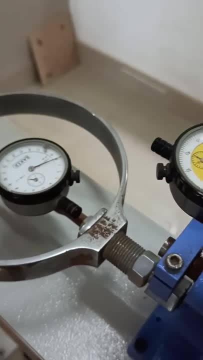 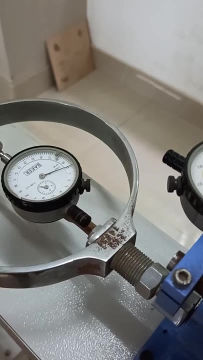 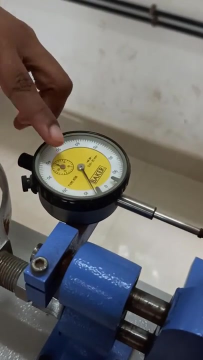 on every 20 divisions, you should read what is the corresponding number of divisions by which the needle of the proving ring is moved. Okay, that is how we take the measurements. Okay, I am now starting the apparatus. So you can see the dial gauge is moving very fast. 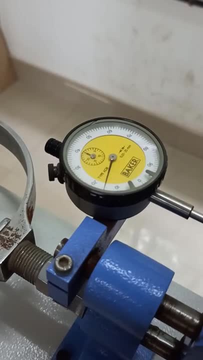 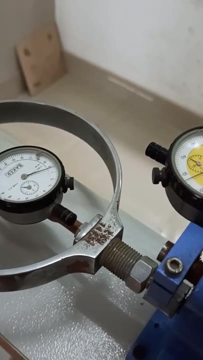 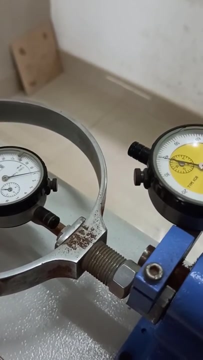 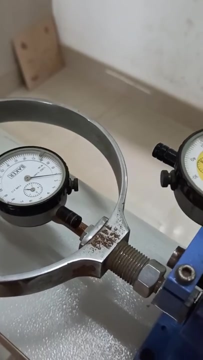 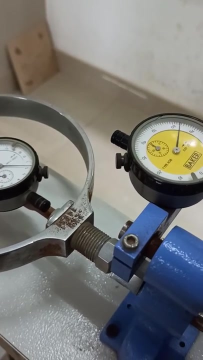 When it reaches 20, read the proving ring. So the number of divisions of proving ring multiplied by the corresponding least count will give the horizontal force which is applied. So you have to take the dial gauge readings or we have to take the readings till the specimen. 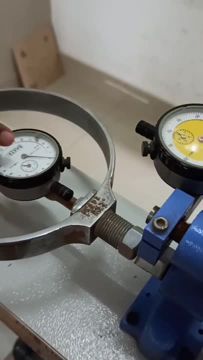 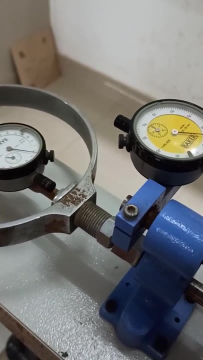 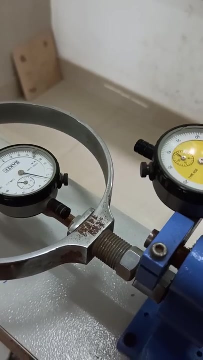 has failed. If specimen fail, you can see the proving ring will start moving reverse. That is how we determine if the specimen has failed or not. Otherwise, if it is not failing for a large extent, you should continue this experiment till 20% of strain has occurred. 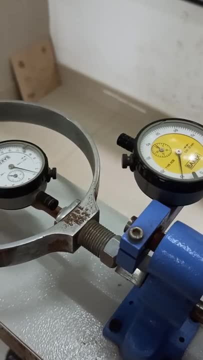 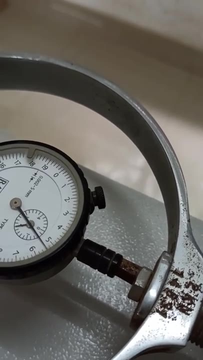 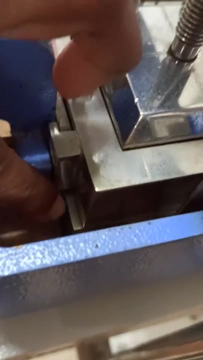 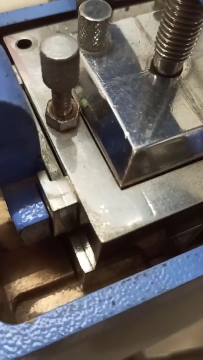 Okay, Now the proving ring has started moving backwards or reverse, So that indicates a failure. Here you can see after failure. you can see this two upper plate and lower plate of the shear box has separated. It is not exactly one over the other. 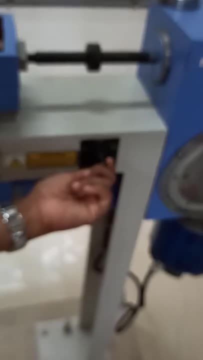 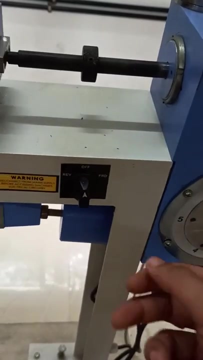 And after this you can turn this knob to reverse mode So you can see the two upper plate and lower plate of the shear box has separated. It is not exactly one over the other. Okay, And while when you turn this to the reverse mode, this shear box will adjust to the initial 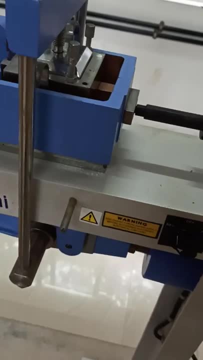 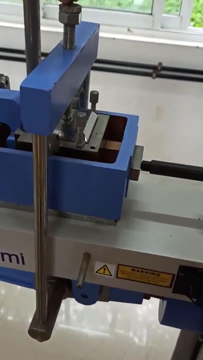 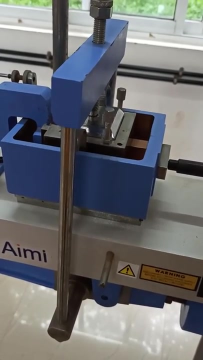 position. And finally, when it has reached to the initial position, the apparatus will stop by itself, and then you can release the screw here and take back this shear box. And then you fill the shear box again with soil and test this for a different normal.